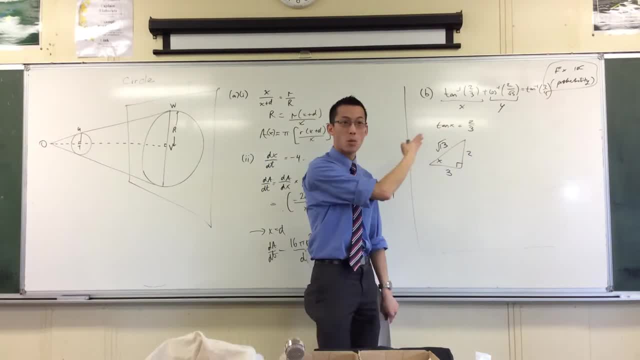 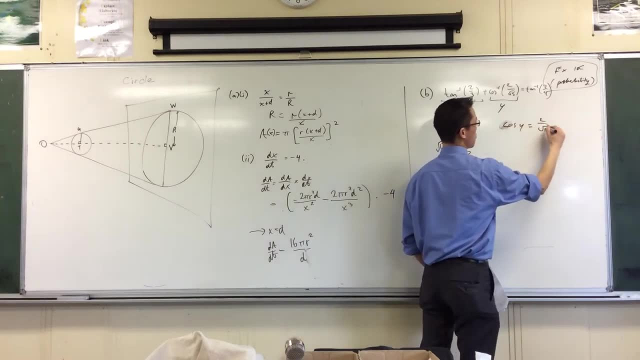 13.. Okay, so there's one of the angles I'm going to need and then over here I can say: well, sorry, not tan, cos y is equal to 2 on root 5.. So you've got your triangle. you stick y over here, so adjacent on hypotenuse. 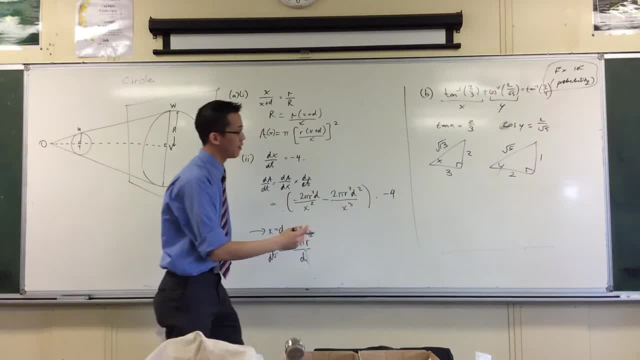 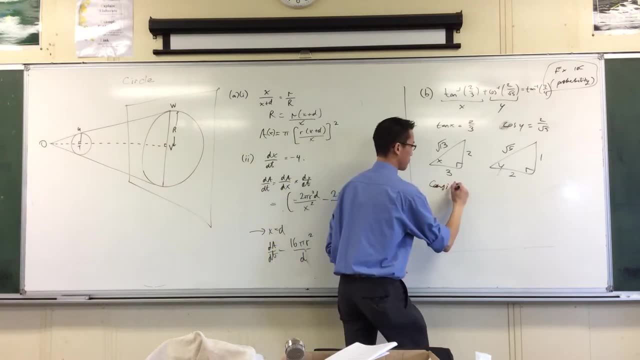 which gives you 1 over there. yes, Okay, so now you can consider right. So this is your starting point. now You can say: consider tan of x plus y right. So you can consider tan of x plus y right. 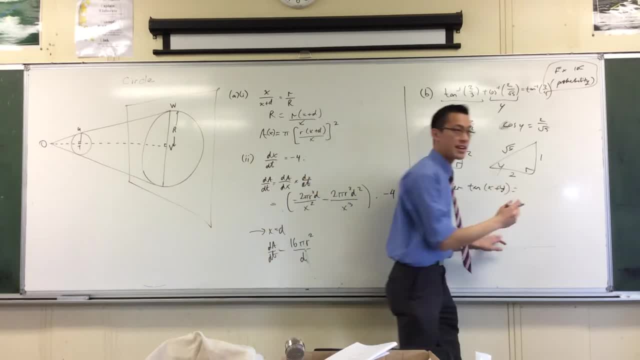 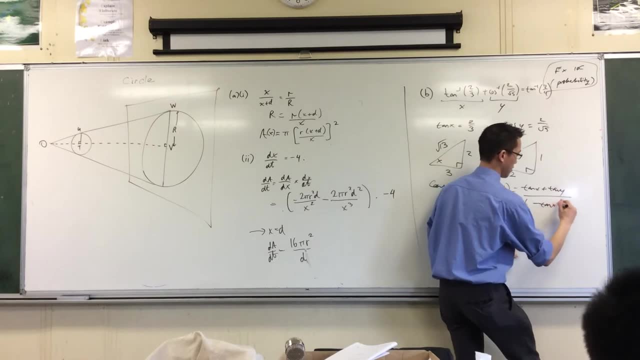 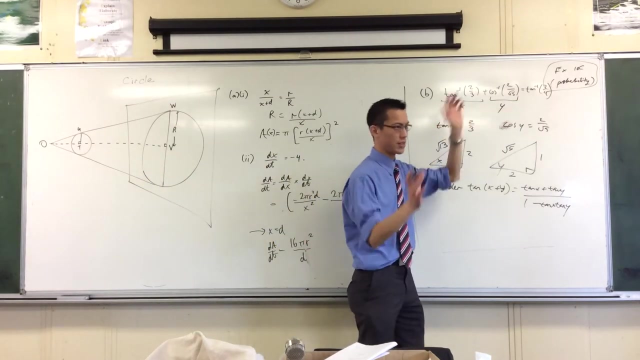 So because they're angles, you can just consider this as the expansion Really really easy. So this would be tan x, tan y, 1 minus Okay. So this is by far the easiest way to harvest it out rather than trying to do tan of cos inverse anyway. 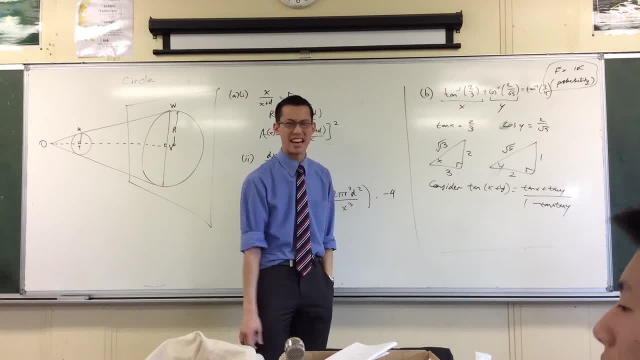 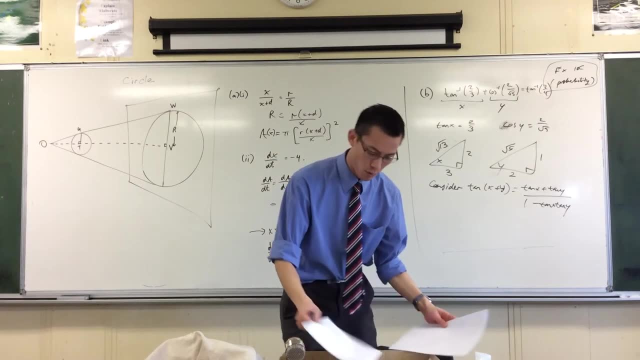 It did work, but I think this is much more straightforward and much simpler, And it's not like it took you a long time to do it either, okay, So once you read it off all out of here, you ended up with the right fractions. 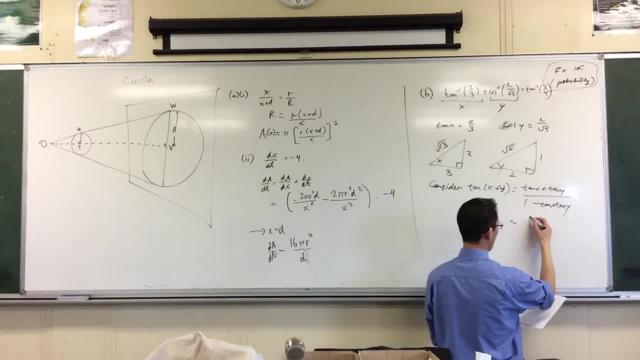 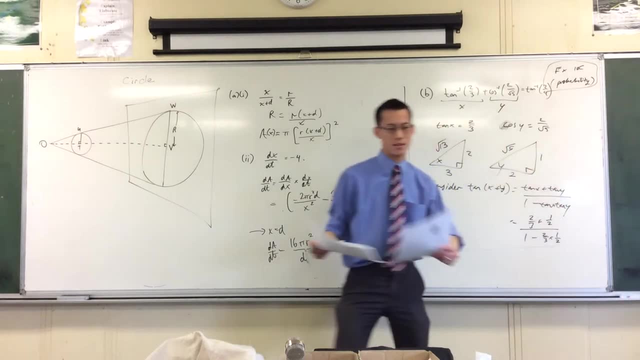 Excuse me, 2 thirds Now. by the way, just as a side note, this is a prove question, right? Sure, Just like so many of them are. there are three marks devoted here, So you can't simply say at this point: 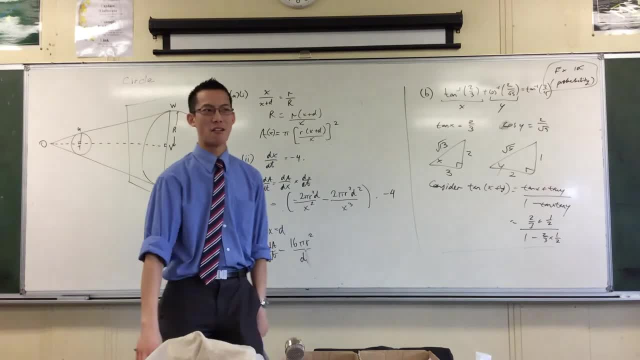 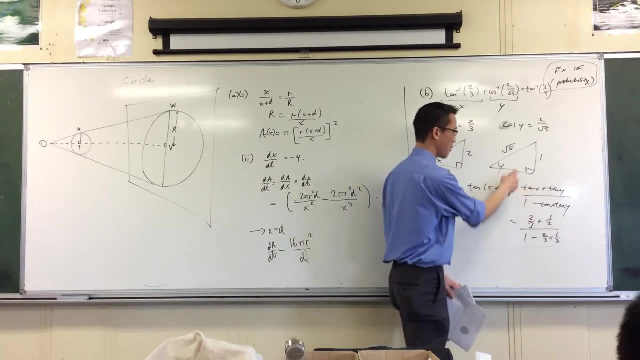 I know this is going to be 7 over 4.. Even though it is right, That's cheating, You have to show it, okay. So this line here is critical, to actually show that I know where all of these come from and I read them off, these triangles. okay, Then it does simplify. 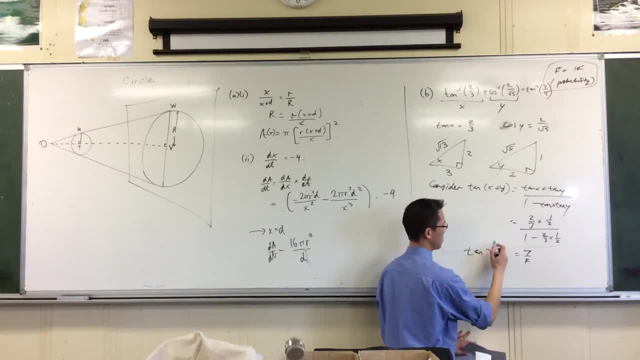 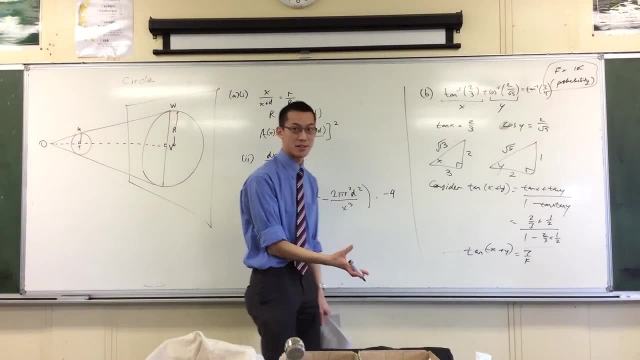 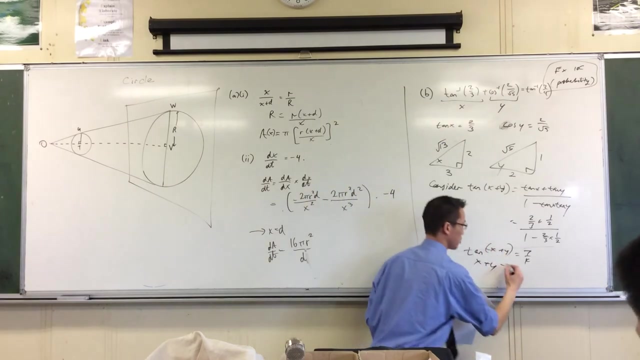 out tan, oops, right, And so now you can take tan inverse of both sides. tan inverse of both sides, okay, On this side, you just get x plus y, which is this, and then on the right hand side, you'll just have tan inverse of 7 over 4, which is what you needed, right. 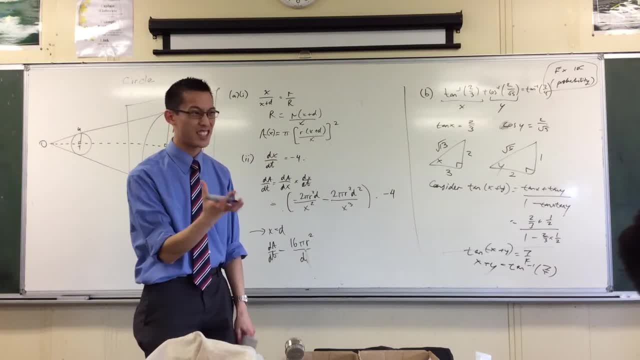 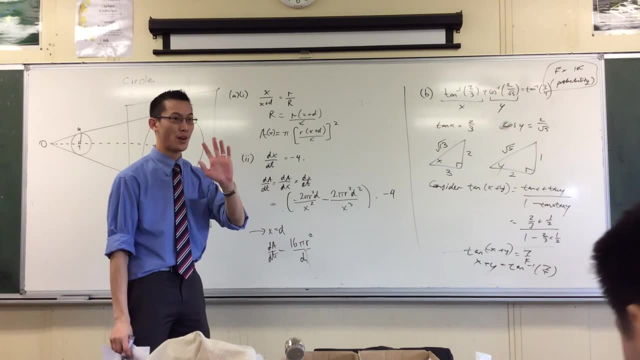 So can you see, even though the maths like the crunching, ends up much the same, your starting point, something like this, sets the solutions apart. okay, It sets apart the people who know what they're doing and the people who are struggling and think: hmm, 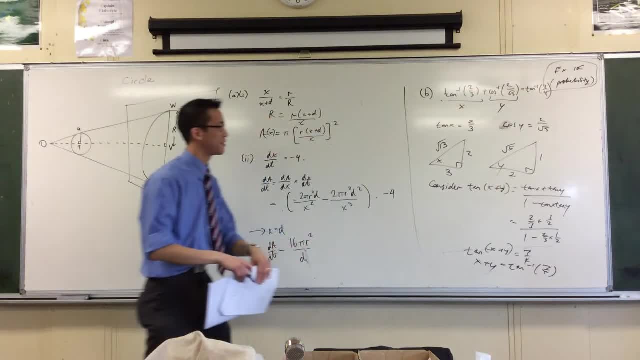 what can I do with this? I know I'll just okay, so watch out for that.